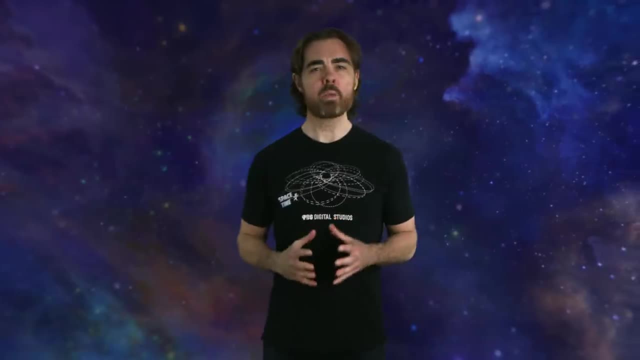 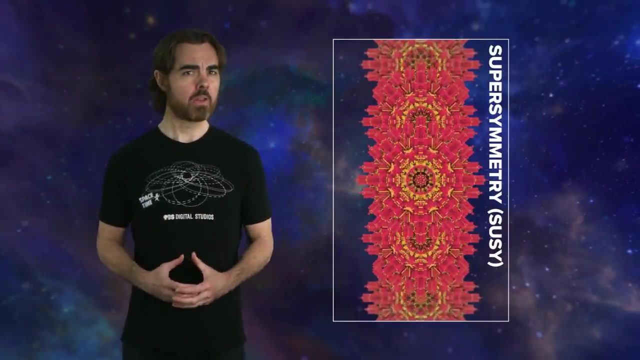 the tiniest hint of new physics from the LHC. One potentially very important ingredient for grand unification theories is supersymmetry. This is one that physics has never seen before. In fact, it's been a long time since physics had really hoped to nail down with the Large 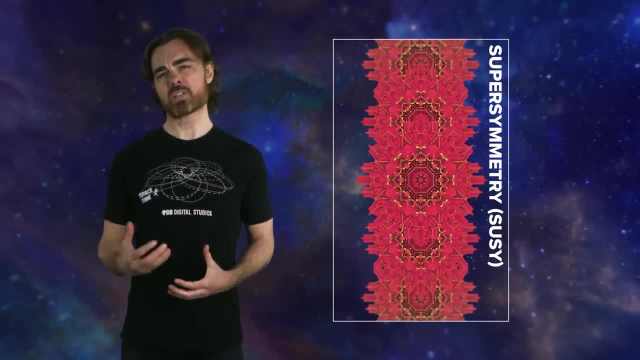 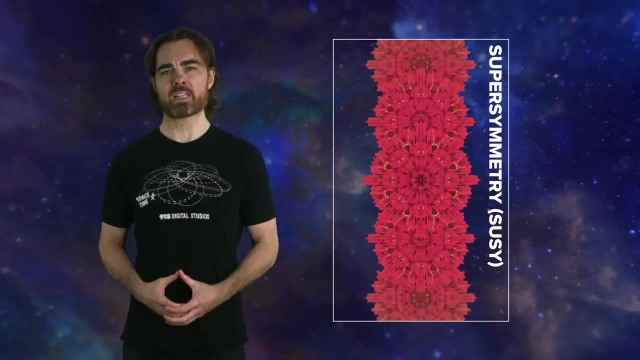 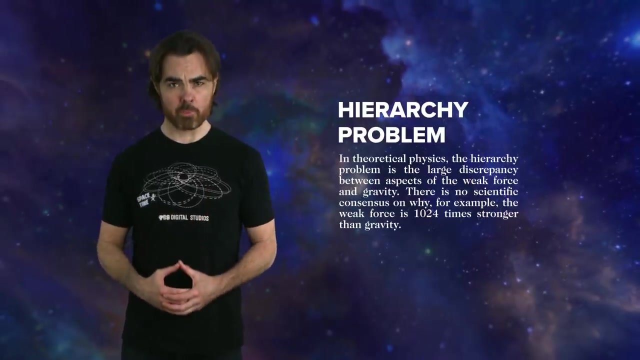 Hadron Collider. SUSY is a proposed extension to the standard model, designed to fix certain issues with the theory, The most serious issue being that the standard model can't explain the minuscule weakness of gravity compared to the other three forces. This is the hierarchy problem. SUSY provides a very natural explanation for the discrepancy. 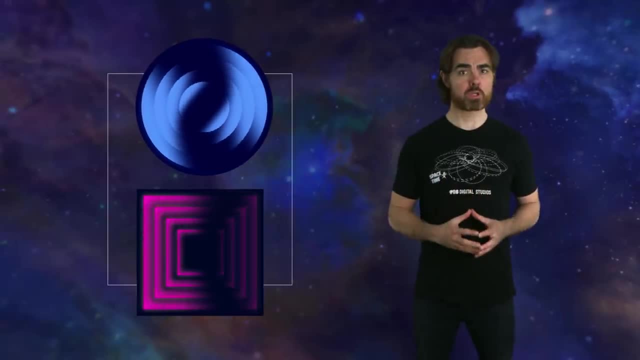 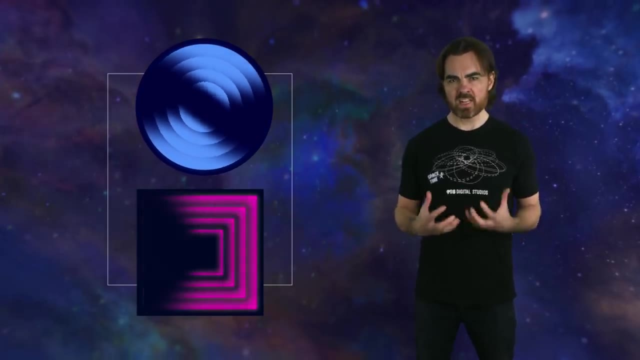 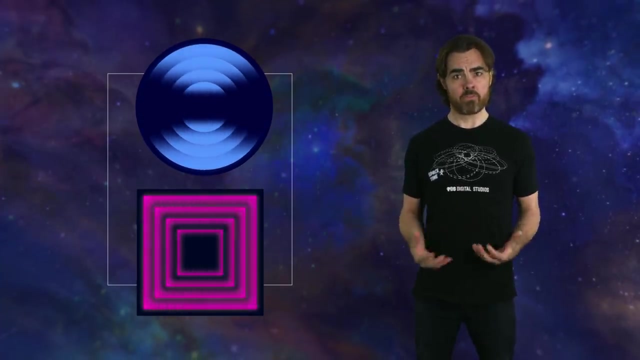 by introducing a new symmetry between the fermions which comprise matter and the bosons which communicate the fundamental forces. As well as fixing the hierarchy problem, this connection between fermions and bosons is, in general, a step towards unifying the particles of the standard model. It's a key feature. 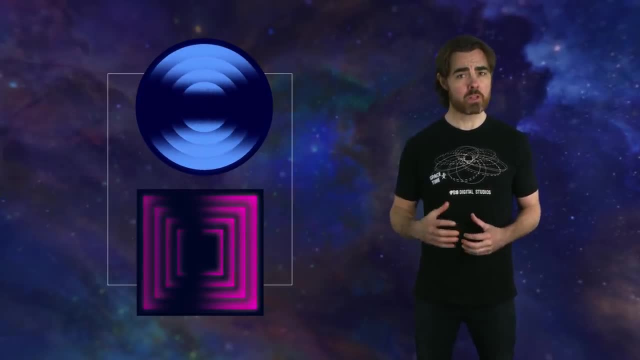 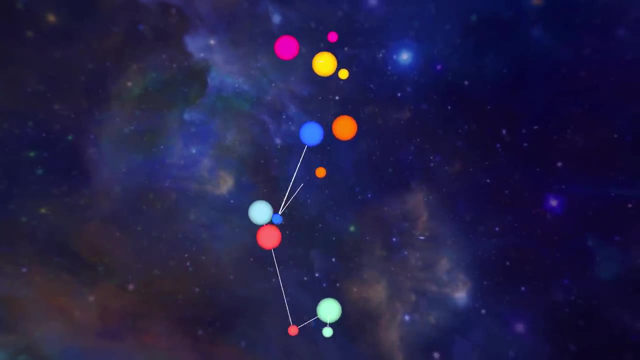 in some grand unified theories as well as modern string theory, levelling it up to superstring theory. Supersymmetry predicts that every single standard model particle has a supersymmetric partner particle of the opposite type. The partners of fermions are bosons and the partners 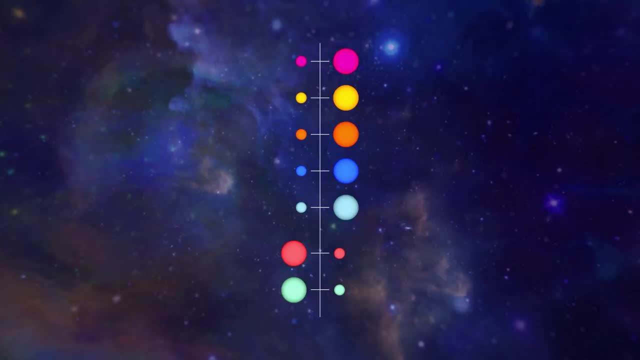 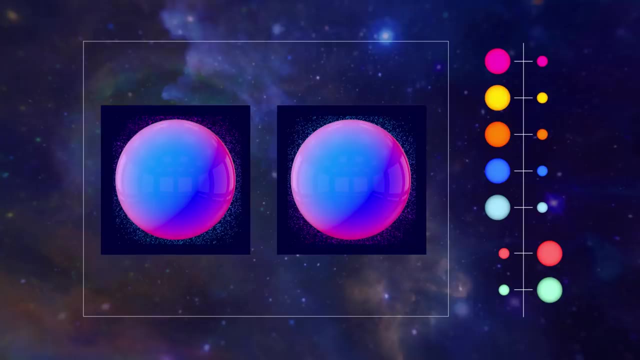 of bosons are fermions. We'll come back to all this in detail another time, but the one property that's relevant for today's episode is that these supersymmetric particles are all expected to be way more massive than their known partners in the standard model. 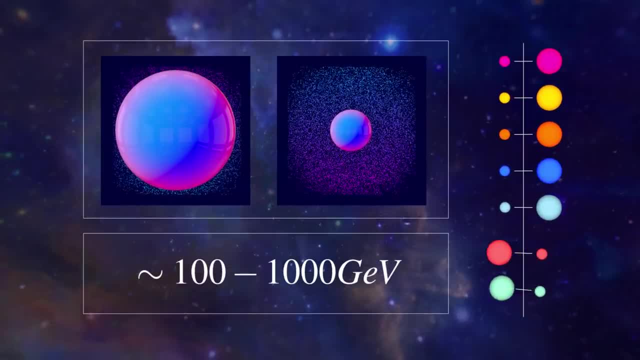 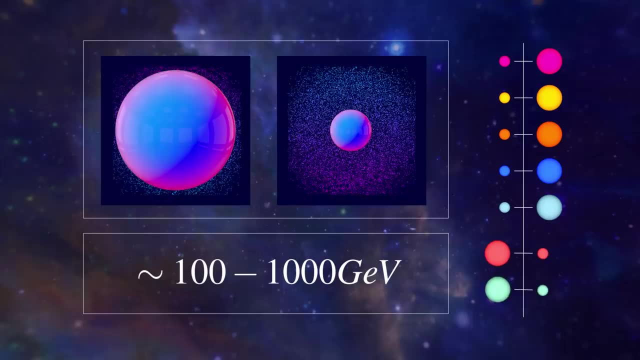 To solve the hierarchy problem perfectly, those particles would need to have masses at around what we call the electro-weak energy, That's the energy at which the electromagnetic and weak nuclear forces merge into the same force. Physicists had hoped that this was. that by smashing particles together hard enough in the Large Hadron Collider there'd be enough energy in those collisions to produce a supersymmetric particle, And in fact there should have been, at least for the versions of SUSY. that most neatly solve the hierarchy problem. But the LHC has seen nothing. This doesn't necessarily kill supersymmetry. It may just be that these new particles are way more massive than expected. If so, they can still help with the hierarchy problem, though not as neatly as we had hoped. 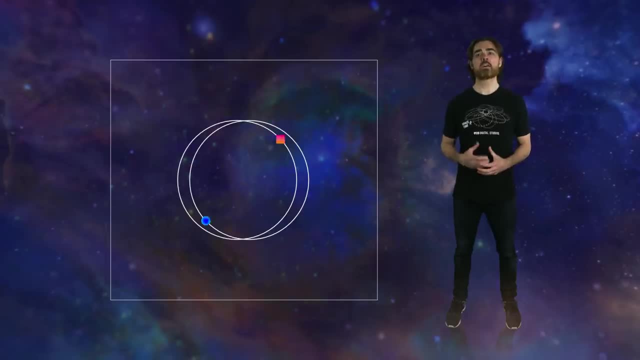 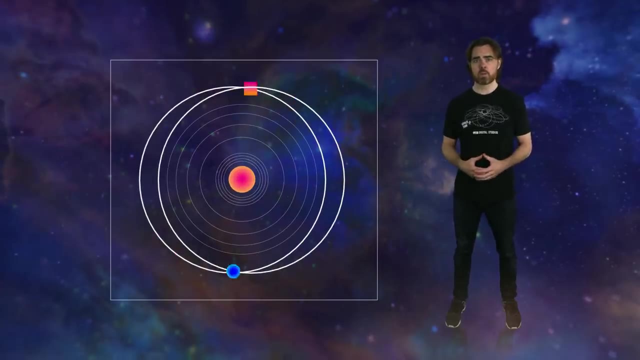 To detect more massive supersymmetric particles you need higher energy particle collisions. So what? build an accelerator the size of the planet, The solar system. Give up and let theorists just tell their stories. Actually, there is a way to probe energies far higher than is possible with the Large Hadron Collider. 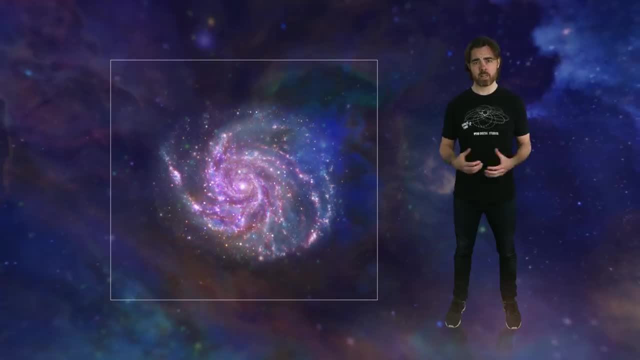 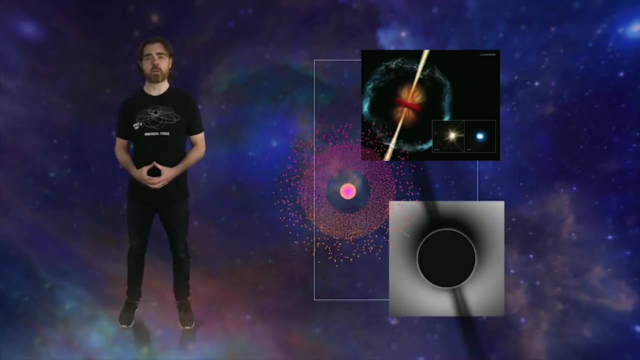 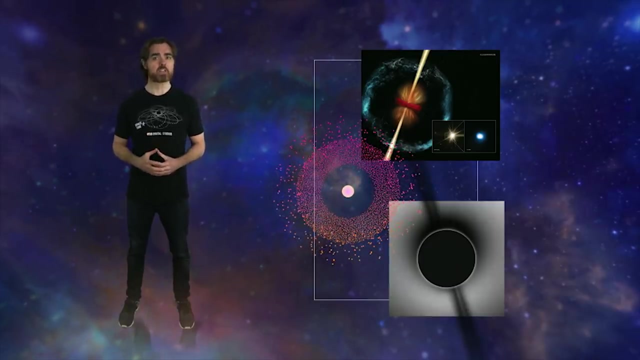 The universe itself is a pretty good particle accelerator. Supernova, explosions, gamma ray bursts, black hole, magnetic fields are all expected to blast high energy particles like electrons and atomic nuclei into the universe. These are cosmic rays. The highest energy cosmic rays can have energies around. 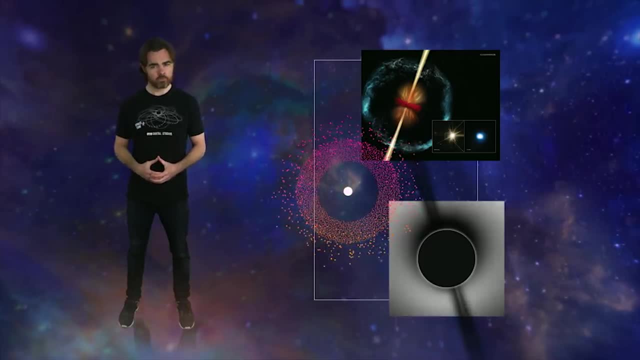 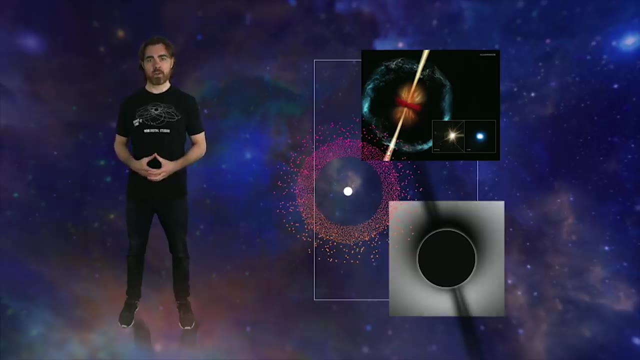 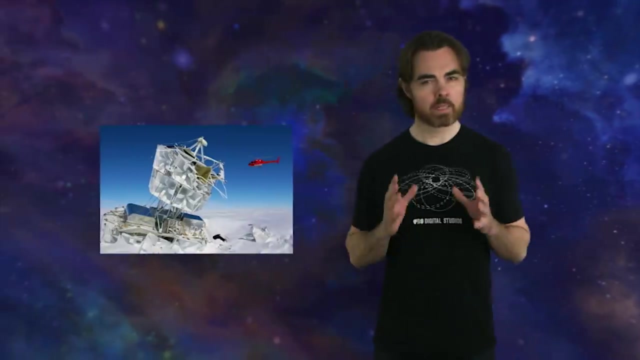 a billion times that of the LHC. Unfortunately for particle physics experiments, cosmic rays at these energies are extremely rare, So it's not surprising that we haven't seen supersymmetric particles in our cosmic ray observations yet, Or have we? Let's talk about this thing. 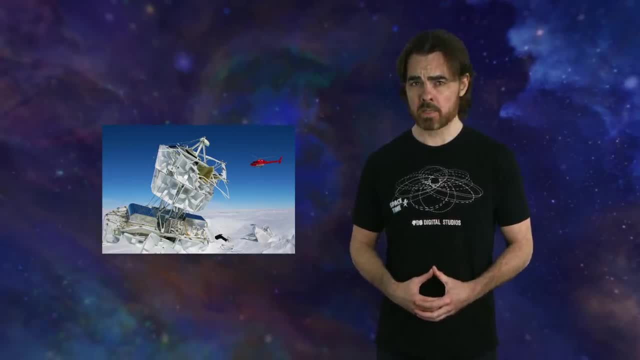 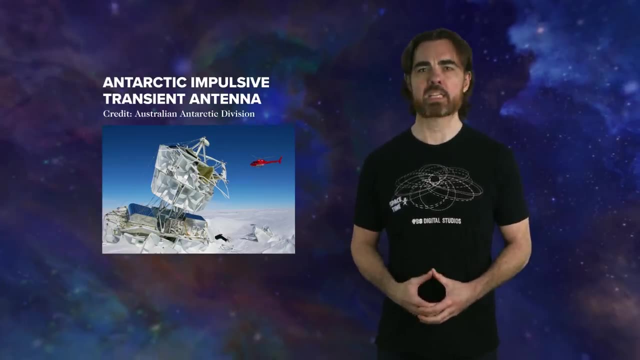 No, it's not a downed imperial probe, droid, Your rebel base is safe. This is ANITA, the Antarctic Impulsive Transient Antenna. It's a cosmic ray experiment of a very special sort. In fact, it's a cosmic ray detector disguised. 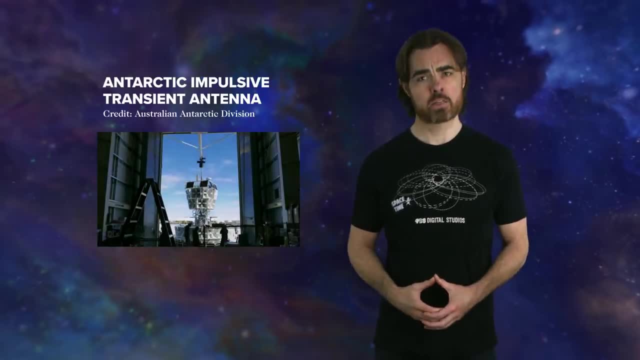 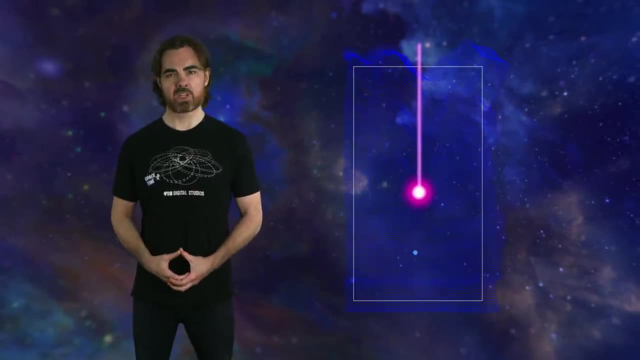 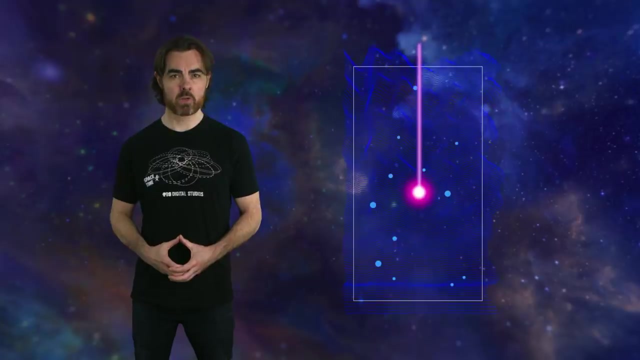 as a neutrino detector, disguised as a radio antenna, disguised as a hot air balloon. Probably I should explain that When ultra high energy cosmic rays travel through space, they bump into the LHC The photons of the cosmic microwave background, That's the leftover heat glow of the very early universe. 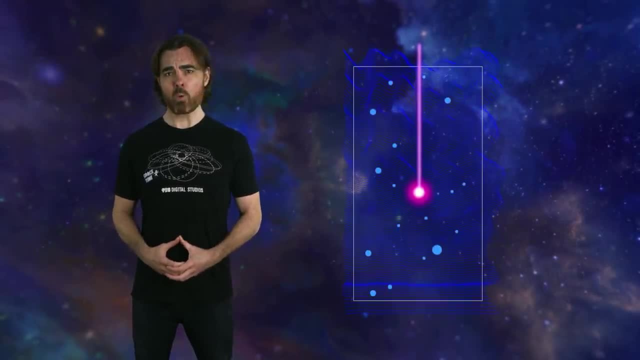 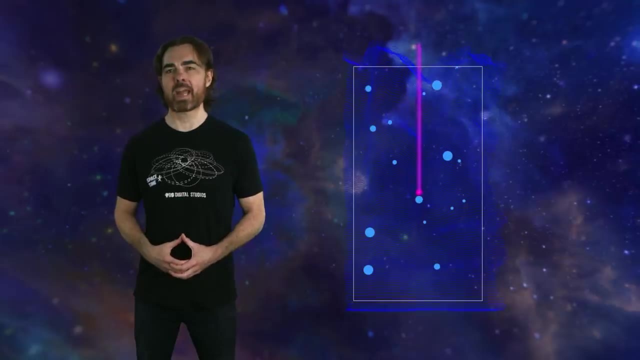 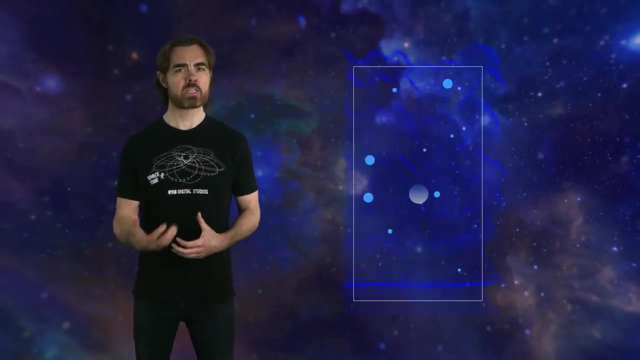 Those cosmic rays lose energy to the CMB, which is partly why the most energetic cosmic rays are so rare here on Earth. But in those interactions cosmic rays can create extremely high energy neutrinos. Neutrinos are almost ghost-like particles that travel through the CMB unimpeded. 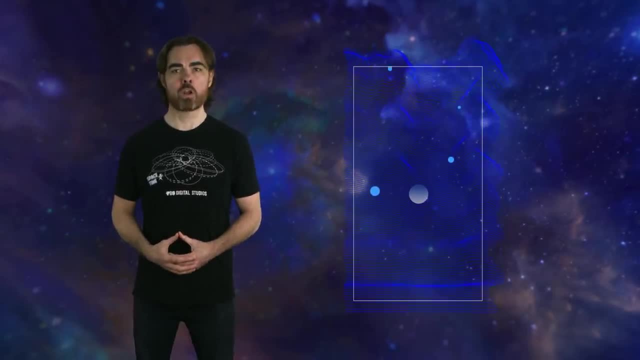 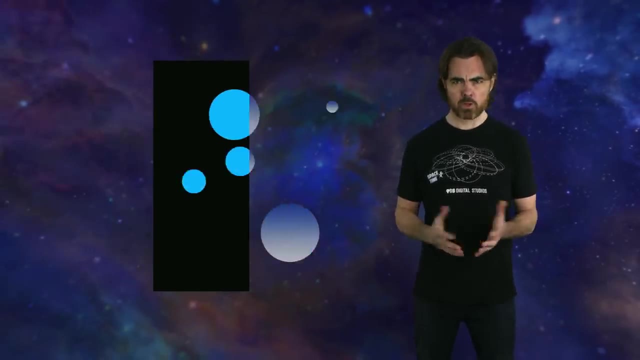 So detecting the highest energy neutrinos allows us to learn about the cosmic rays that produce them. These neutrinos don't just ignore the CMB. They can pass through solid matter. Lower energy neutrinos can flow right through the Earth as though it isn't there. 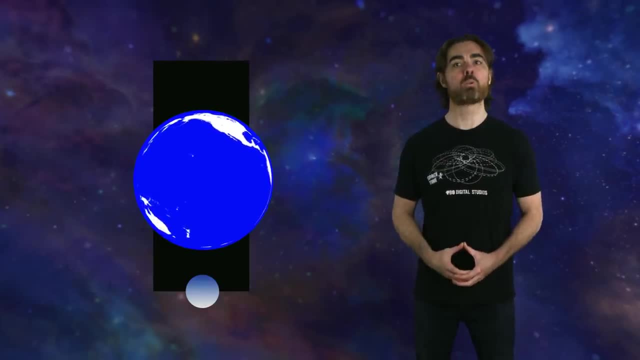 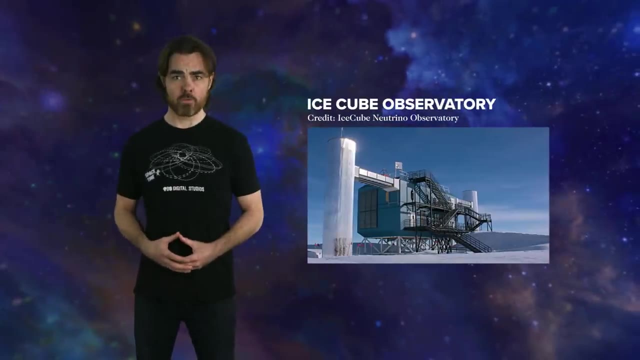 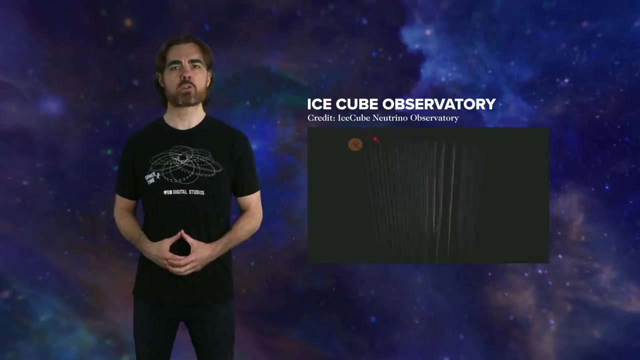 We detect neutrinos because very, very rarely one will interact with an atomic nucleus and produce a shower of particles. For example, the IceCube Observatory is a one kilometer cube of the Antarctic glacier laced with photon detectors. It spots neutrinos. 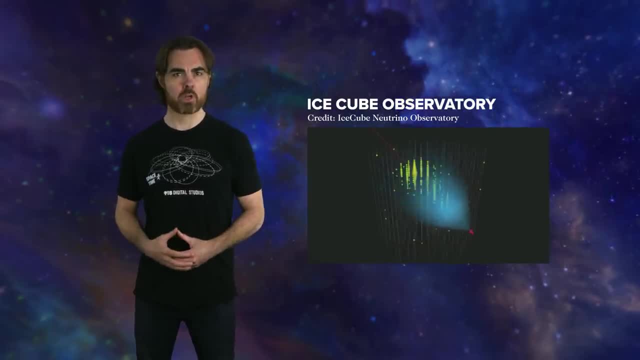 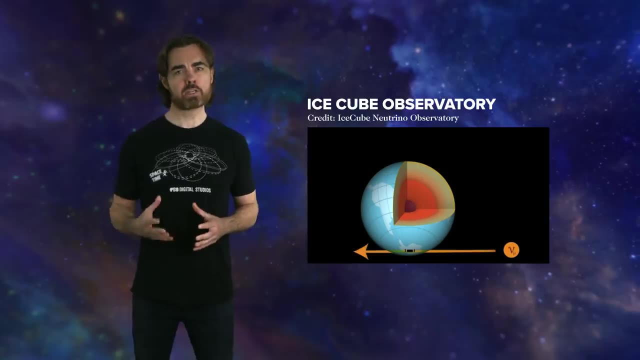 When they decay into electrons, muons or tau particles, which in turn produce visible light as they streak through the ice. This is Cherenkov radiation, and IceCube's photo detectors track these flashes. ANITA works in a similar way, but it's. 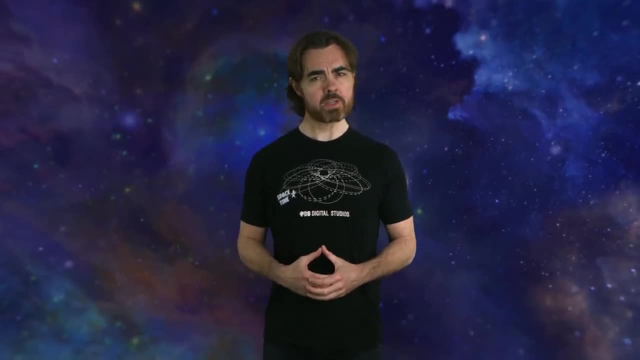 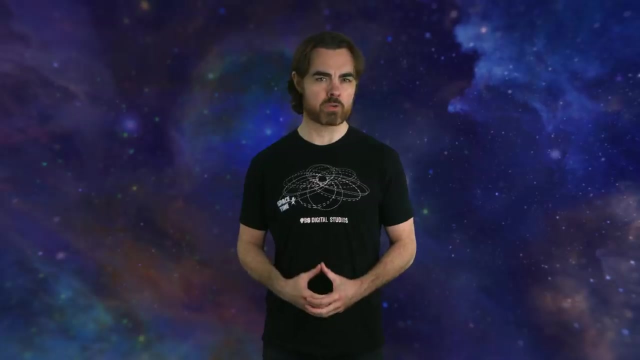 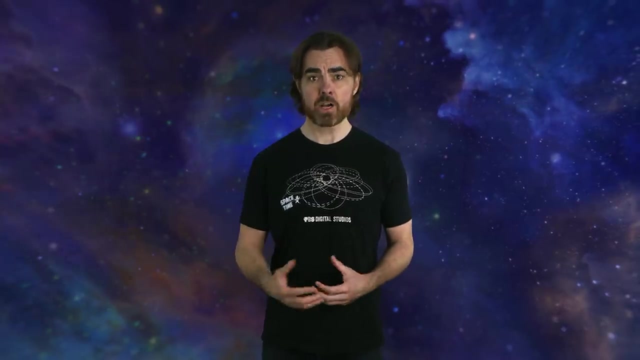 focused on catching the very highest energy neutrinos, the ones that are produced by cosmic ray interactions with the CMB. In order to see those extremely rare neutrinos, ANITA scans not one cubic kilometer of ice, but 15 million square kilometers of Antarctic ice sheet. 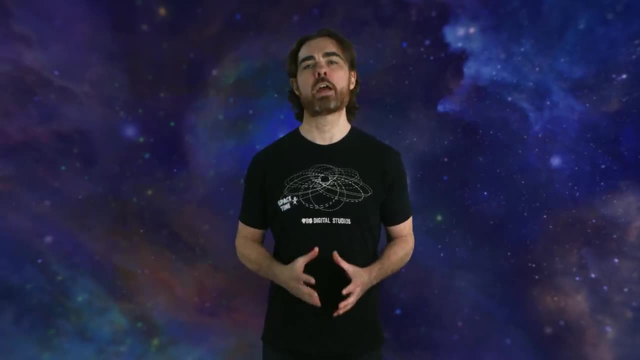 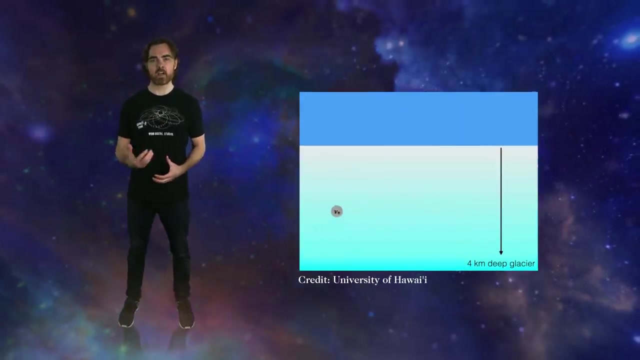 That's where the balloon comes in. ANITA is a cluster of radio antennae that hovers 37 kilometers above Antarctica. If an ultra high energy neutrino decays in the ice anywhere within 700 kilometers of ANITA, the resulting radio frequency Cherenkov. 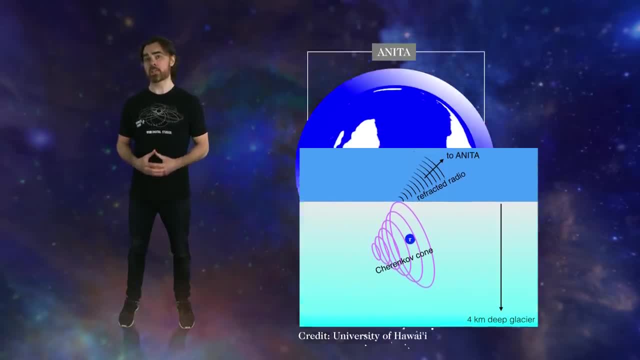 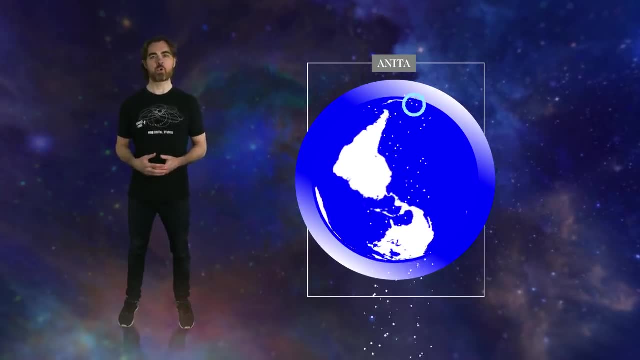 can be seen by ANITA's antennae. ANITA is designed to detect neutrinos that are coming from below, passing through the ice, through the Earth, into the ice sheet. That allows it to sort out neutrino radio flashes from the flashes produced. 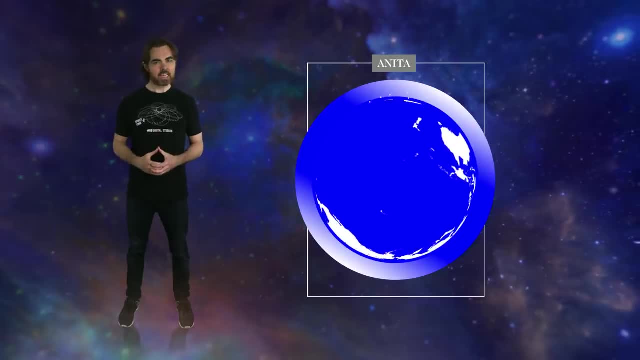 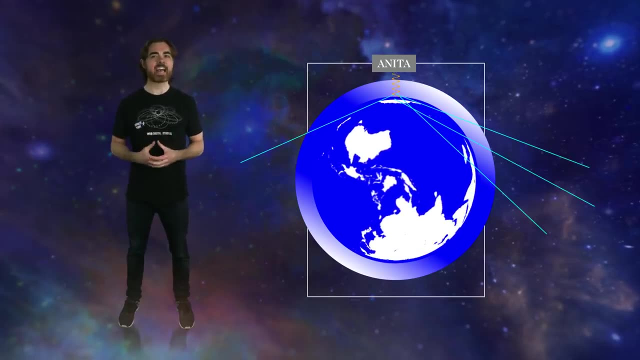 by other cosmic rays coming in from above. In fact, ANITA expects to see its most interesting, most energetic neutrinos coming in at an angle skimming the arc of the Earth on a shallow trajectory. They should not come from directly below. 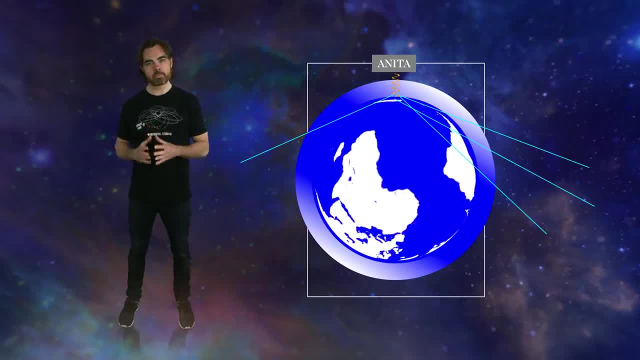 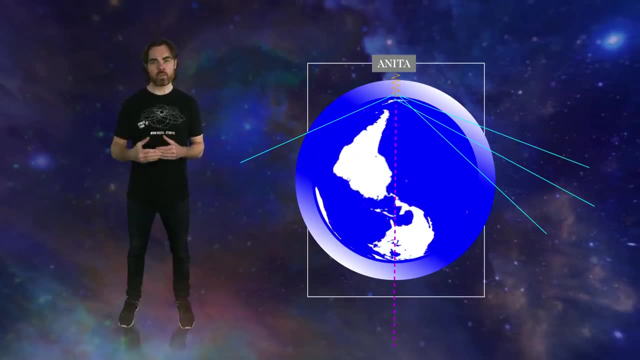 which would require them to pass through the entire planet. That's because the most energetic neutrinos actually do lose energy If they're passing through the Earth. they aren't expected to make it all the way through without slowing down significantly. So you can imagine that ANITA scientists were a little. 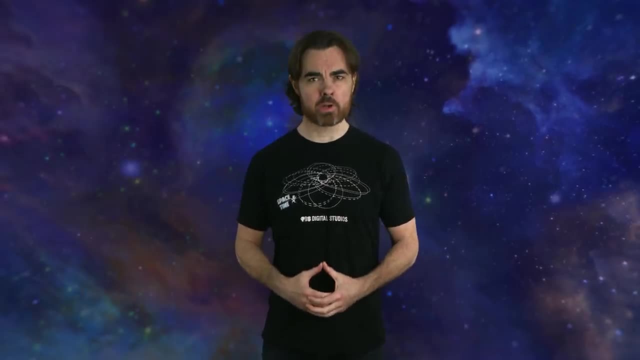 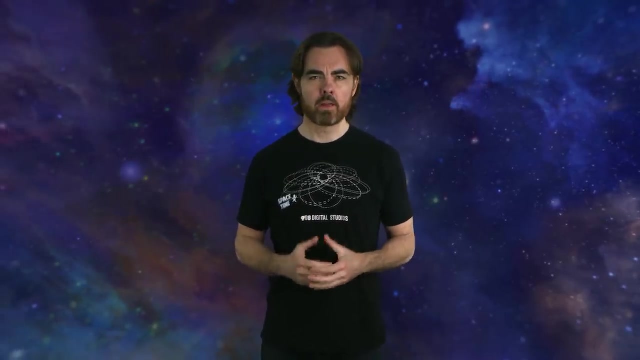 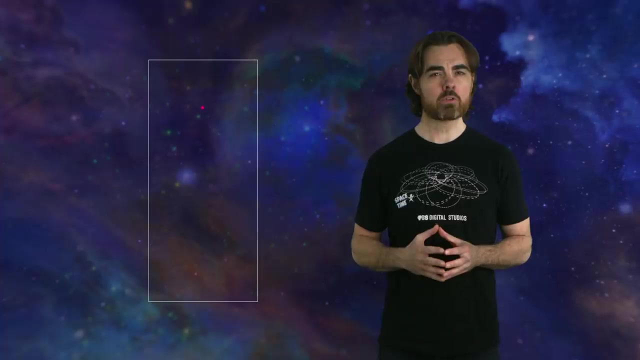 confused when they spotted two extremely high energy radio bursts that could only have been produced by a high energy particle, passing all the way through the middle of the planet. That's several thousand kilometers of rock magma and iron, Ignoring the ridiculous distance they traveled. 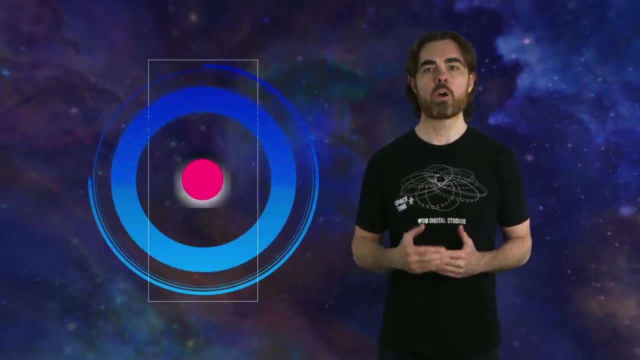 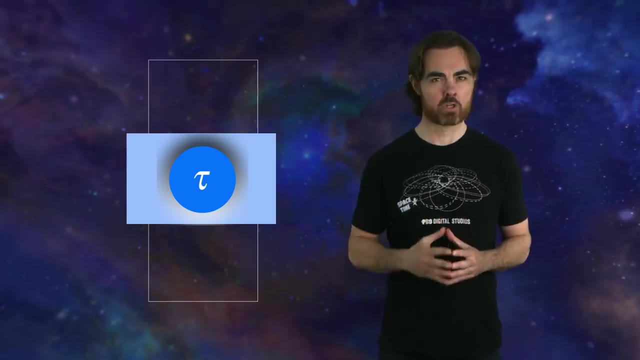 these events look like what you'd expect from a very high-energy neutron, But in reality they're not. The TAU neutrino, a particular flavor of neutrino. the TAU neutrino interacts with the ice and transforms into a TAU lepton. 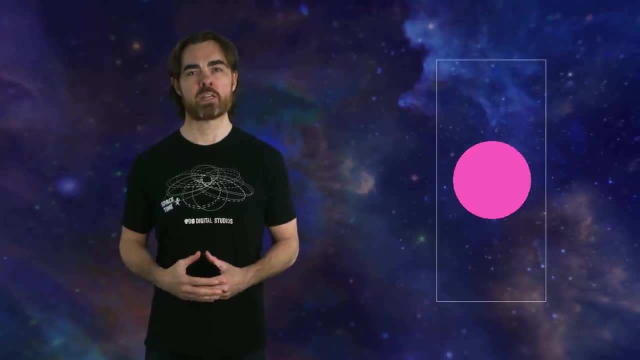 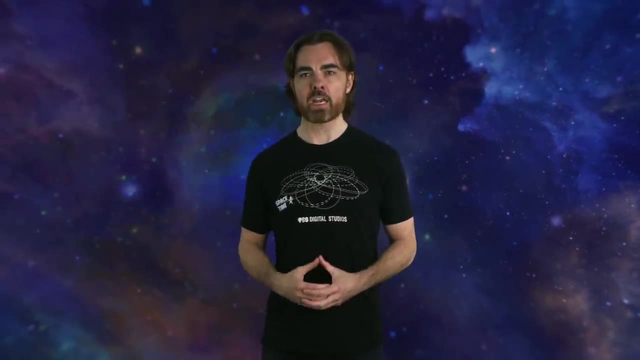 And that's the heavier cousin to the electron. The TAU is cool because it's so short-lived: It produces a Cherenkov burst when it's created and then a second burst when it decays into a shower of secondary particles. But seeing these very high-energy TAU events, 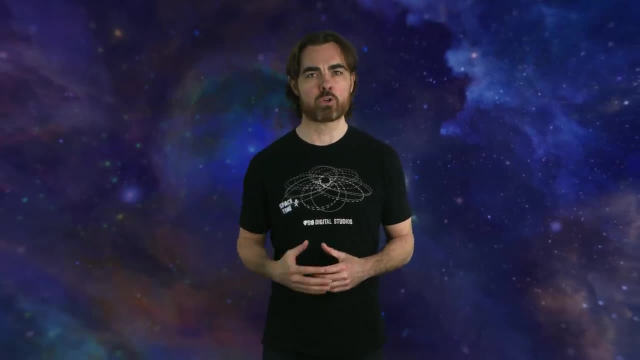 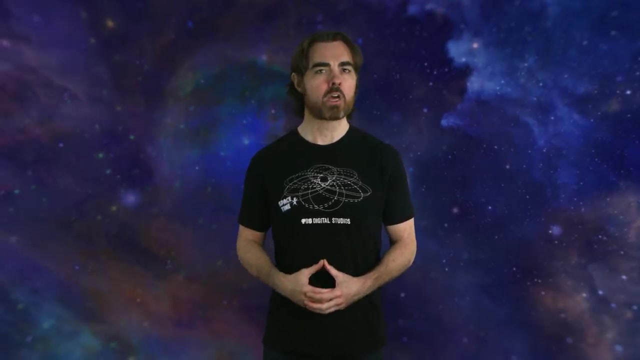 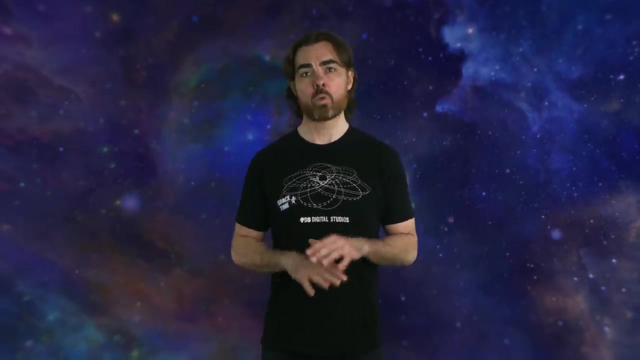 from directly below doesn't make sense. It's estimated that there's around a one in three trillion chance that two TAU neutrinos could have been seen in the amount of time Anita has been looking. Physicists are having trouble accounting for these event. 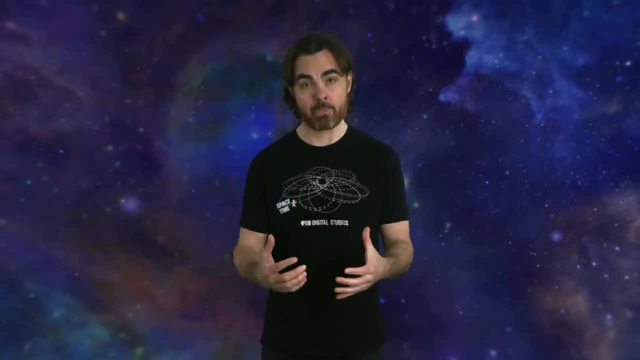 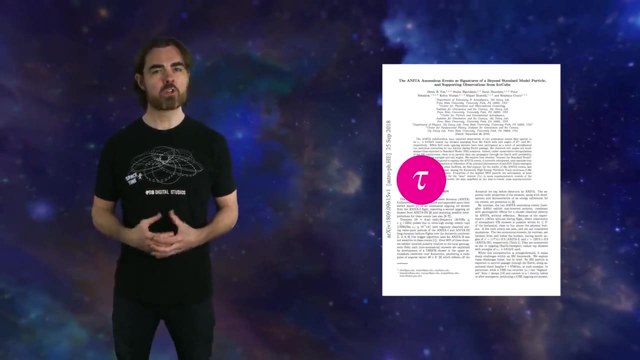 with any known standard model particle, Which brings us back to supersymmetry. Astrophysicist Derek Fox, Stein, Sigurdsson and team point out that there's a version of supersymmetry that predicts exactly the right particle to do this job. 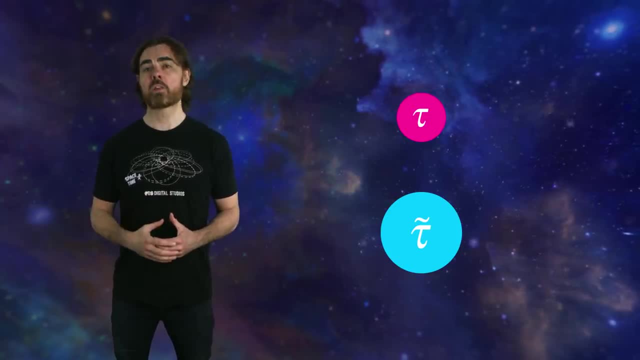 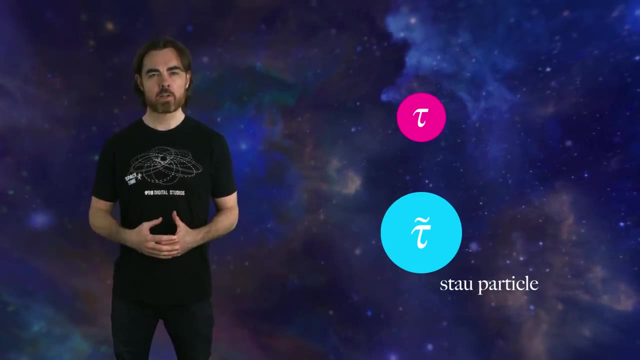 It's the supersymmetric partner of the TAU lepton, the STAU particle. Yeah, you put an S in front to get the SUSY particle, Selectron, squark, STAU. Supersymmetry is super easy. Here's the scenario. 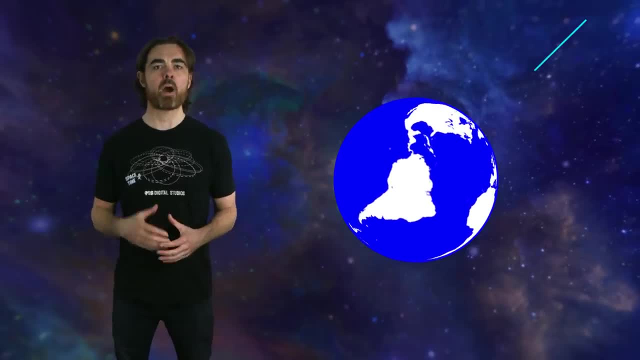 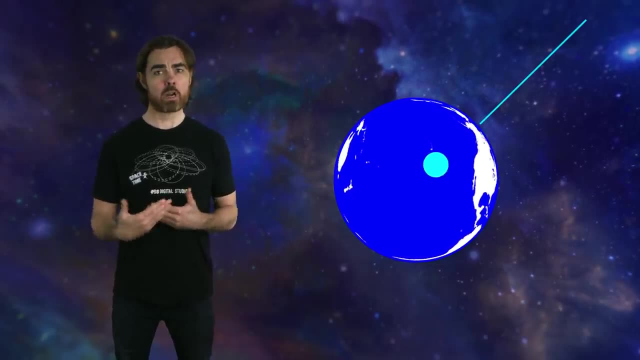 A STAU particle was produced on the opposite side of the planet by an incoming ultra-high energy neutrino plowing into the Earth. The STAU is theoretically capable of zipping straight through the Earth before decaying into a regular TAU lepton on the other side. 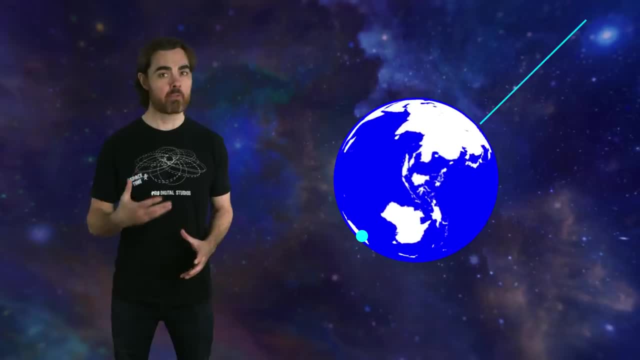 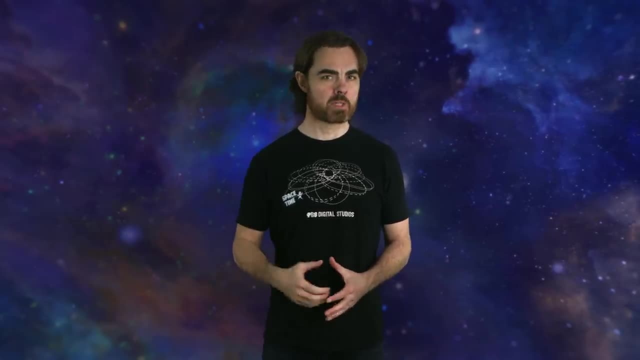 This then causes a high energy radio flash coming from directly below. That's quite a story, but it fits the observations pretty well. There are, of course, other possibilities. It could be a so-called sterile neutrino. Now, we talked about that before. 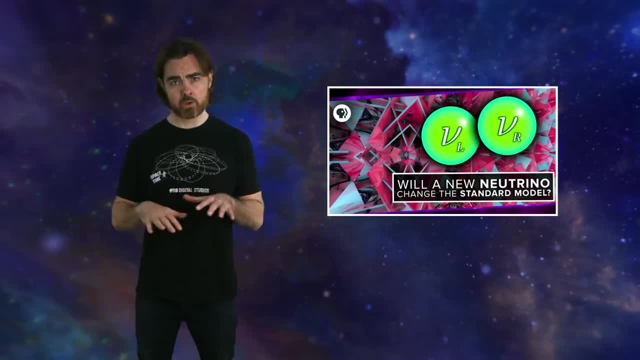 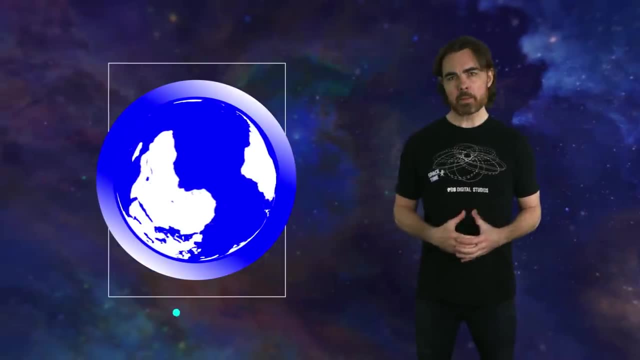 This particle is also not in the standard model, but has nothing to do with supersymmetry. Hints of its existence have been found in the Fermilab particle accelerator experiments. It may also be that there were some gigantic bursts of regular neutrinos at the time of the observed events. 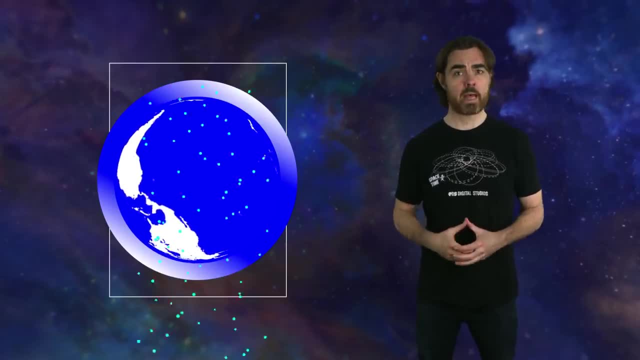 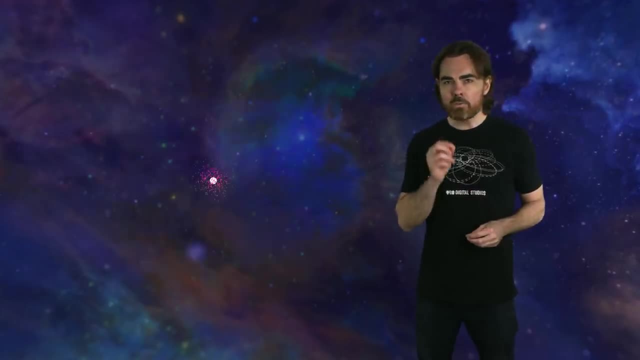 Hit the Earth with enough high energy neutrinos, for example, from a supernova explosion, and at least some of the ultra-high energy ones could make it through. In fact, one of the two events may have been associated with a distant supernova. that 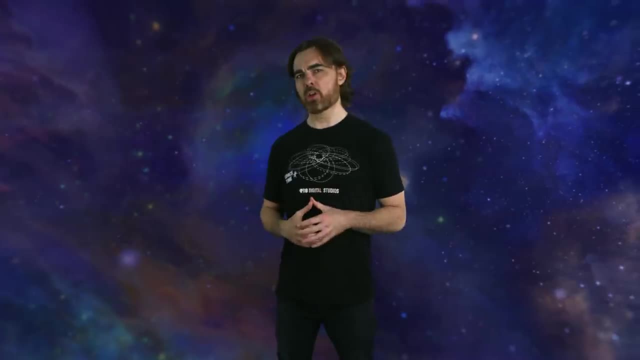 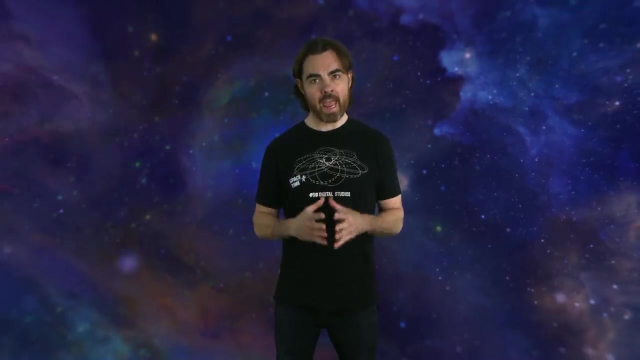 was observed around the same time and location. The probability of a chance association with a supernova is around 3%, so it's unlikely, but it does happen. On the other hand, the supernova is not likely to be observed. The supernova in question wasn't nearly bright enough. to make even one Earth-penetrating ultra-high energy neutrino likely. And remember there were two events at different times. The other event wasn't associated with any supernova or gamma-ray burst. The final possibility is just that we're missing something. 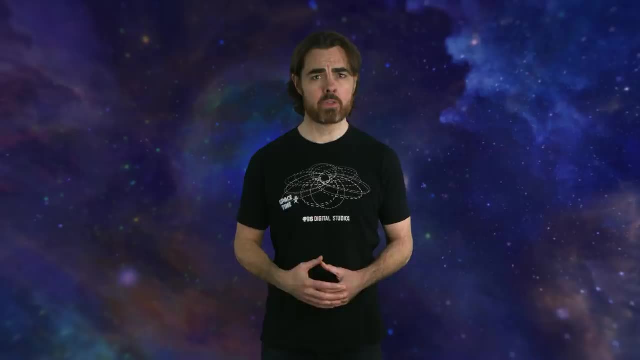 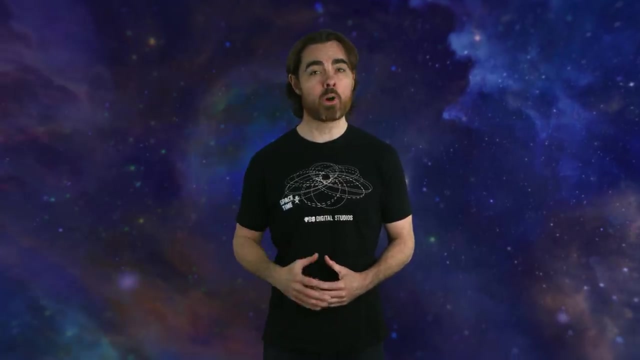 Perhaps our understanding of neutrino propagation through the Earth is flawed, or perhaps penguins use cell phones now. This is going to require a lot of research. It's going to require more observation and confirmation. The first step would be to look at the other big neutrino. 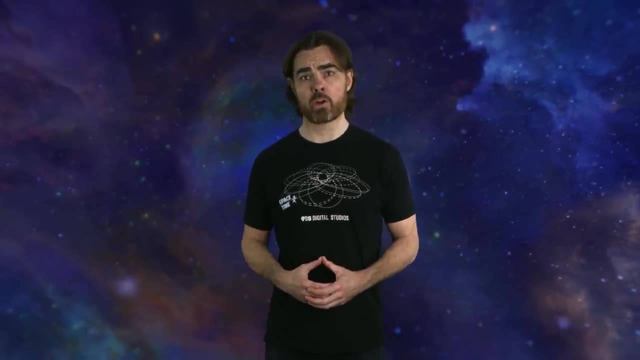 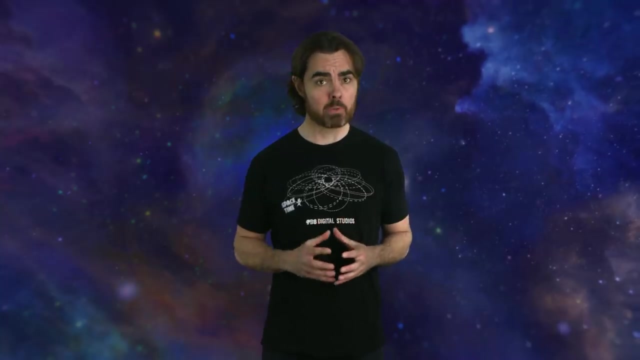 observatories, IceCube is really the only one that could have potentially spotted similar events. Actually, given the amount of time IceCube has been in operation, it probably should have. Fox and team looked back into the IceCube archive and actually did find some possible high energy. 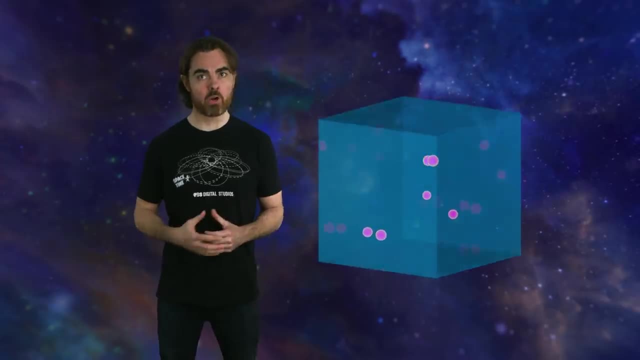 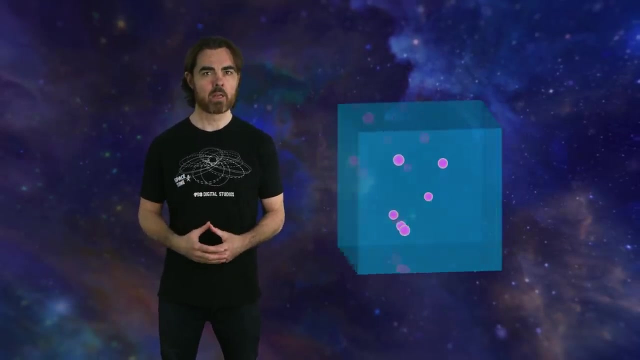 tau lepton events that may have come from directly below. The data is a little ambiguous. They may have been boring old muon neutrinos that can easily pass through the planet, but you can bet people will be paying a lot more attention to these sorts of events from now on. 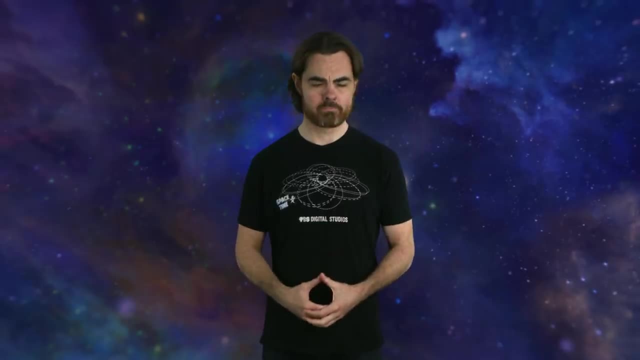 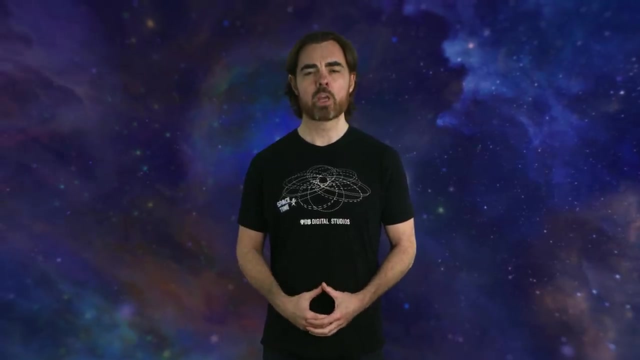 So have we gone beyond the standard model and proved supersymmetry? Hell, no. What we have is a tantalizing hint. Given the painful absence of new particles from the Large Hadron Collider, any hint of something new is bound to get physicists excited. 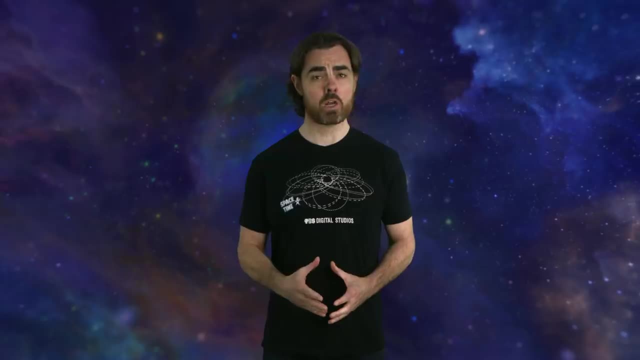 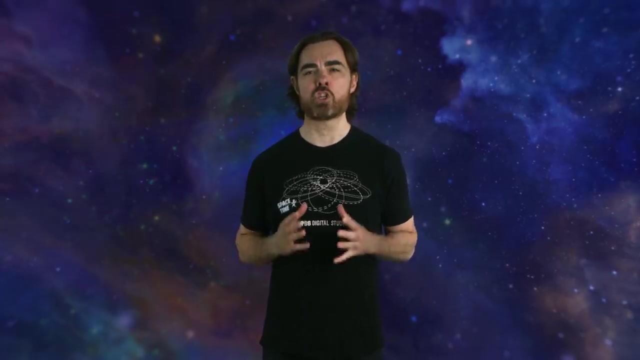 ANITA will keep flying, IceCube will start carefully scrutinizing its data and if these mysterious events from below keep arriving, you can be sure that physicists will find an ingenious way to confirm their nature. Perhaps we'll verify the existence of the stau. 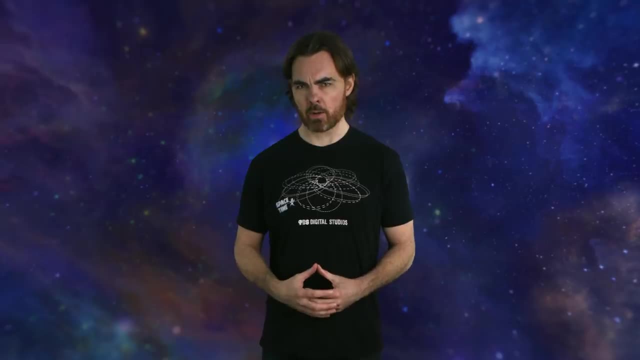 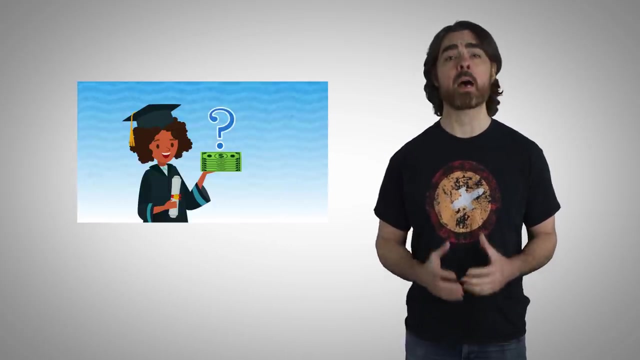 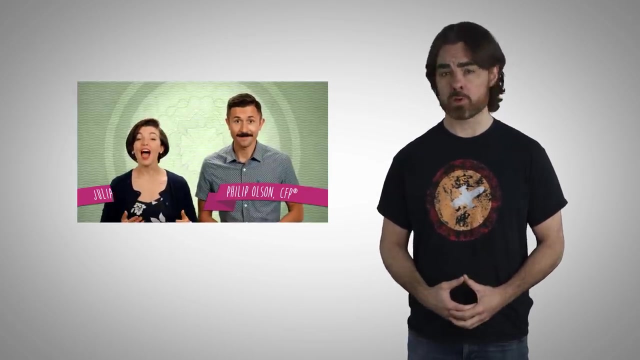 and with it confirm the supersymmetric nature of space-stime. Before we get to comments, I just want to let you know about Two Cents, the PBS digital series about personal finance. Financial experts Philip Olson and Julia Lorenz Olson guide you through the complex world of personal finance. 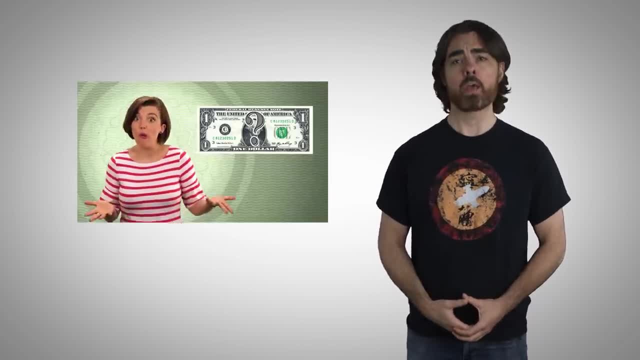 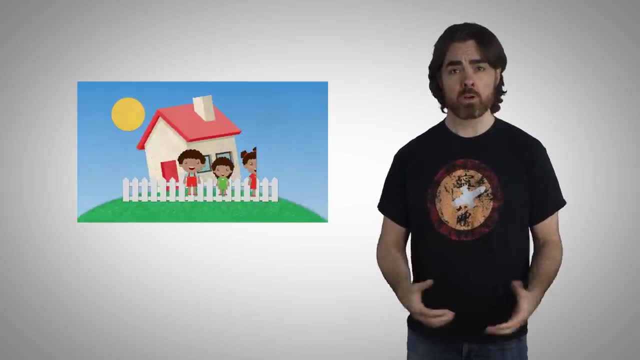 from the kitchen table to the New York Stock Exchange. You'll get practical knowledge about how to spend, save and earn and insight into how your brain is hardwired to react to economic problems. If you have any money and might like to have some more, 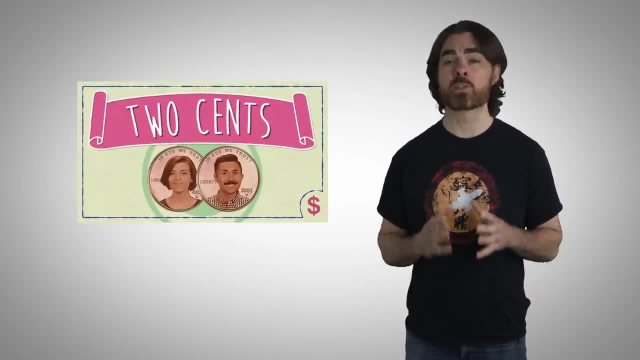 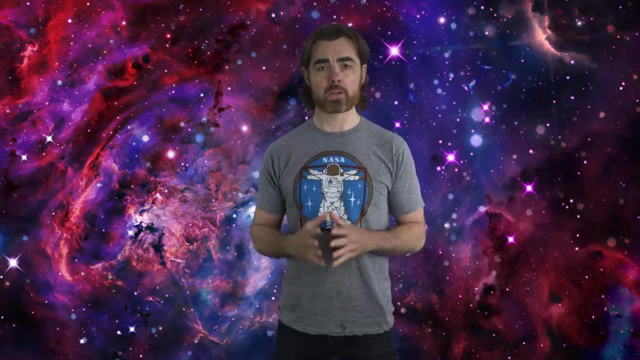 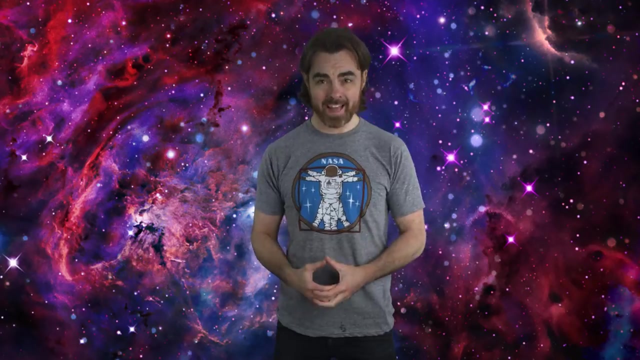 check the link in the description below to subscribe to Two Cents. Last week we talked about why string theory is so compelling to so many physicists. Now, before I get to specific comments, let me address a common objection. Many of you have some interestingly passionate hate. 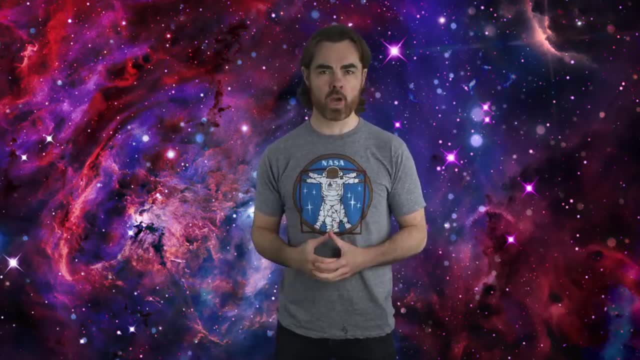 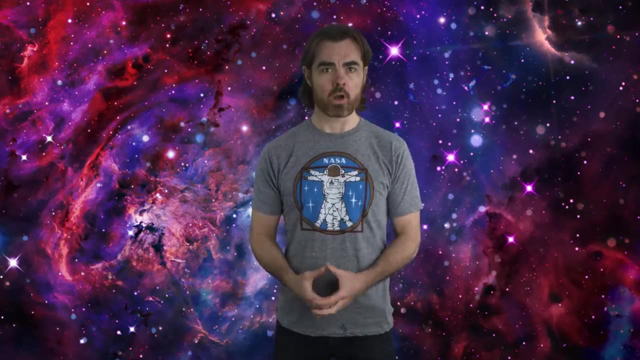 for string theory on the grounds that it's so far proved unfalsifiable. Some of you say that means it's not science. Now I'm not sure. I agree with you. String theory may be wrong, but it's not testable due to the limits of current facilities. 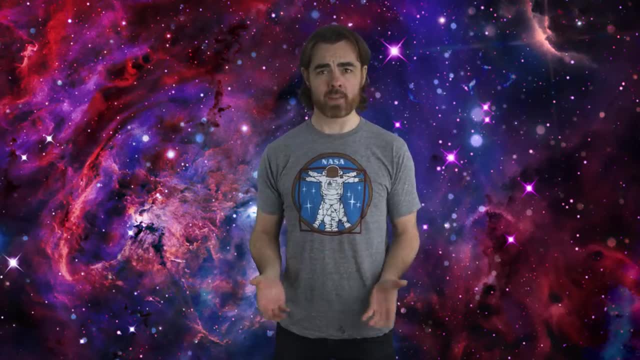 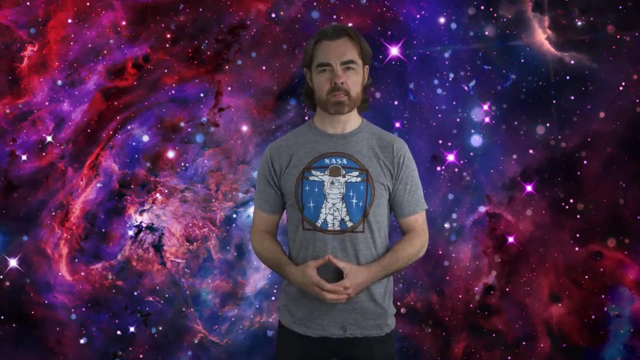 Does that mean it's not science? Well, the universe has no obligation to operate in a way that is currently testable by any particular size particle accelerator, nor does it have any obligation to be simple enough to be deduced by even the smartest primates. 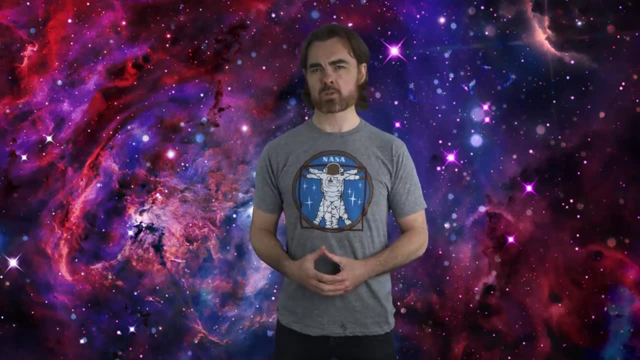 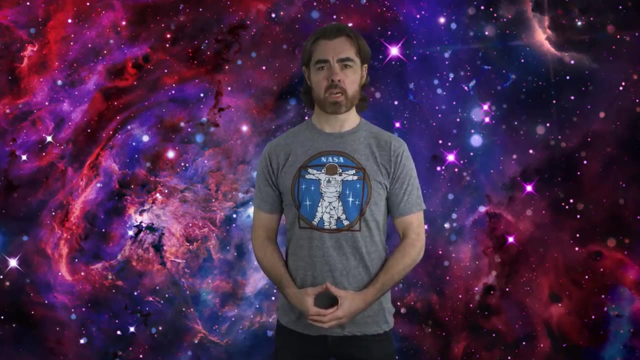 in one generation or in 100.. The thing that makes string theory less sciency is that its modern version, M-theory, is not particularly well-defined, But again, that doesn't mean it's wrong. Wolfgang Pauli's not even wrong might be a better description. 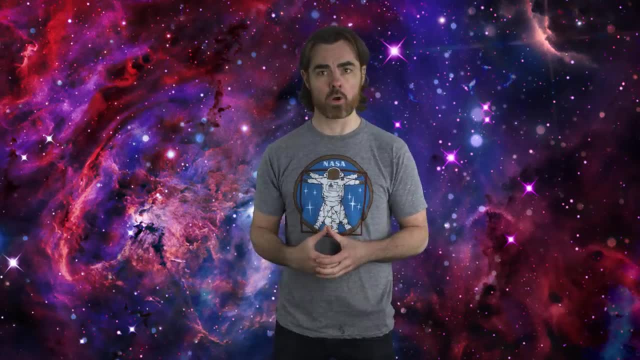 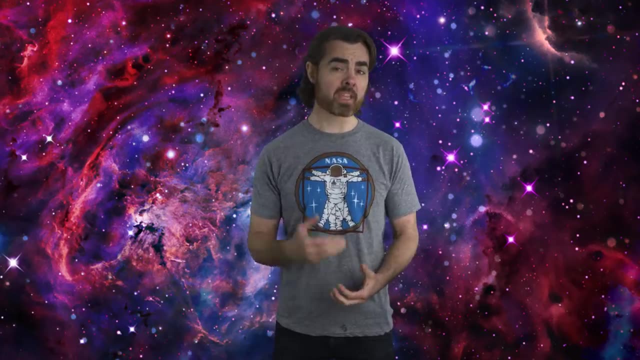 String theory is not precise enough yet to be confirmed wrong, which means it might be right or not. Eddie Galtek asks why you can't get meaningful energy from the, the Casimir effect. Well, it's the same reason you can't get continuous energy. 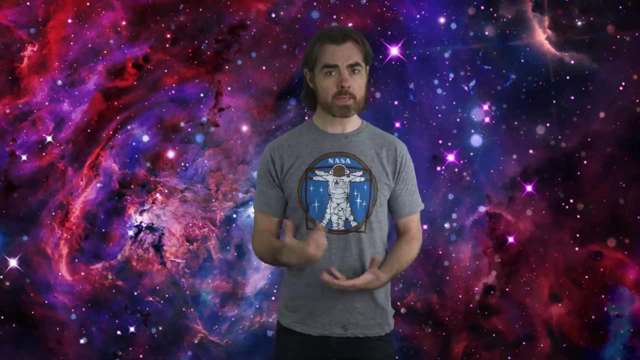 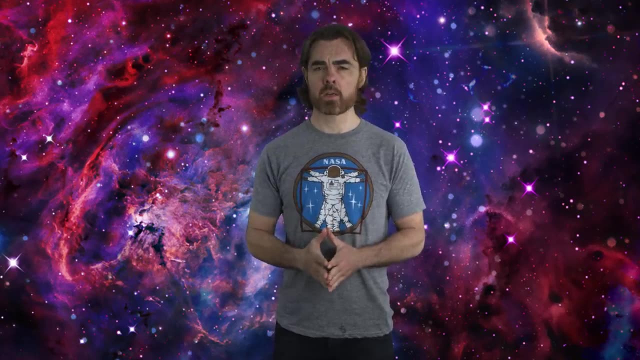 for a ball falling off a roof. You get the kinetic energy once, but then you have to expend at least as much energy raising the ball back to the top of the roof. Same with the Casimir effect: The Casimir plates pull together. 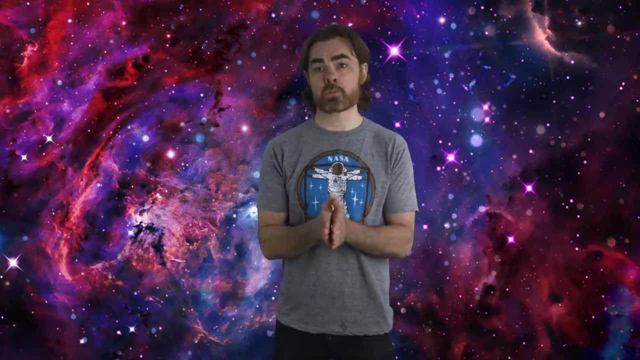 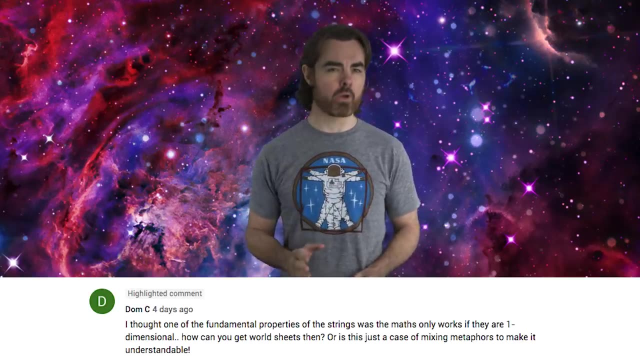 giving you a very tiny amount of energy, But to get more energy you have to pull them apart again, which takes just as much energy as you got when they fell together. Dom C asks a good one To quote, I thought, one of the fundamental properties. 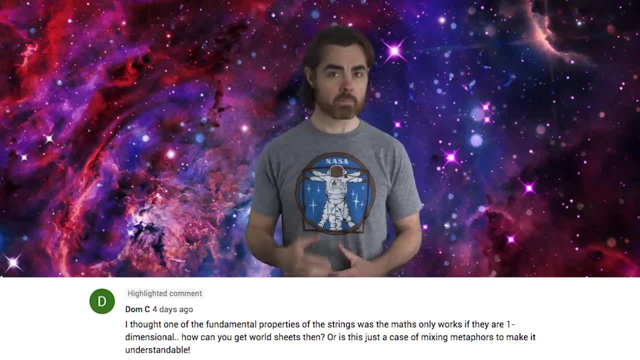 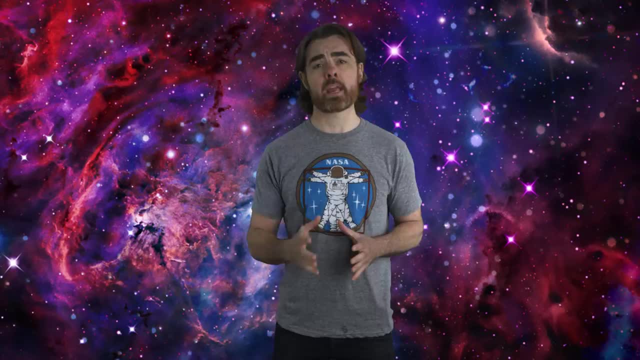 of the strings was that the maths only works if they are one dimensional. So how can you get world sheets? Yes, it is a pain keeping the number of dimensions straight in string theory, While invariance only works for the 2D world sheet, which 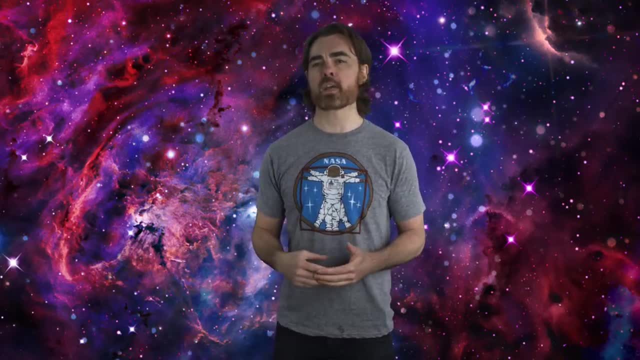 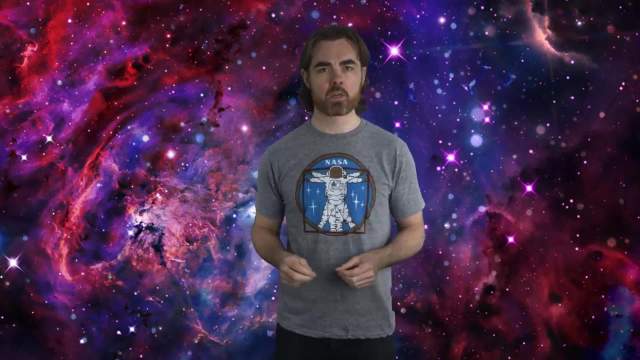 has one dimension of space and one of time. This is the shape traced out by a string moving through time. A 2D world sheet has to be traced by a 1D physical object. So yeah, the math of string theory only works for 1D objects because these trace 2D world. 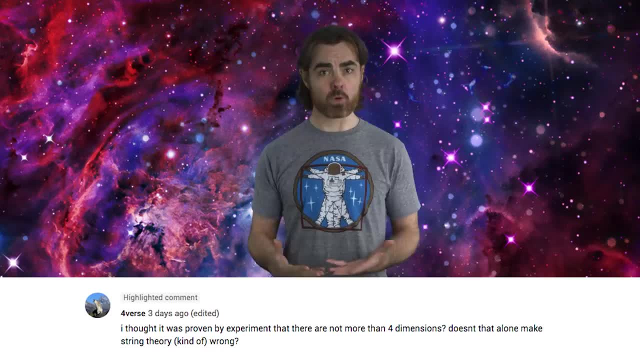 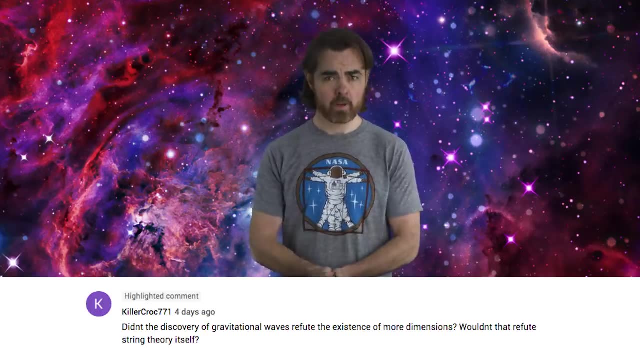 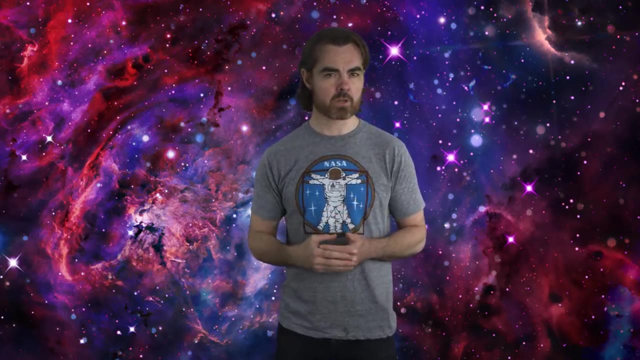 sheets. Some of you recalled a recent episode in which we talked about a study of gravitational waves that appears to refute the idea of extra dimensions. Good memory, Actually, this study was specifically evidence against the idea of extra extended dimensions. One explanation for the unusual weakness.